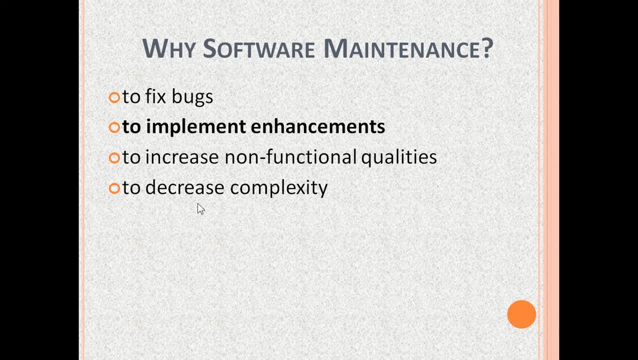 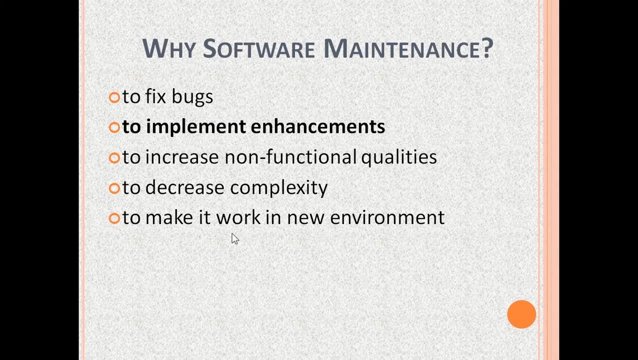 Enhancing the software in these ways- by implementing enhancements, increasing non-functional qualities and decreasing the complexity- is also called perfective maintenance. Software maintenance is also required to make the software work in new environment, like upgraded hardware, new or upgraded operating system, new database management system or other software. 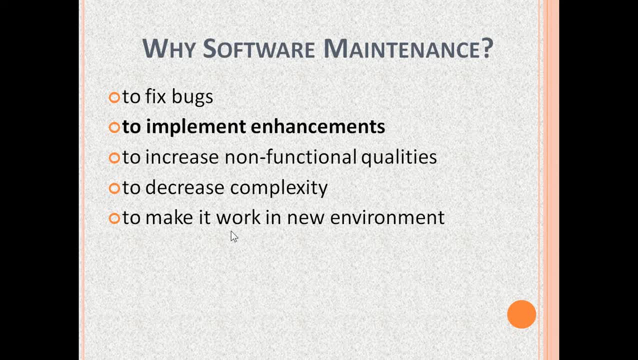 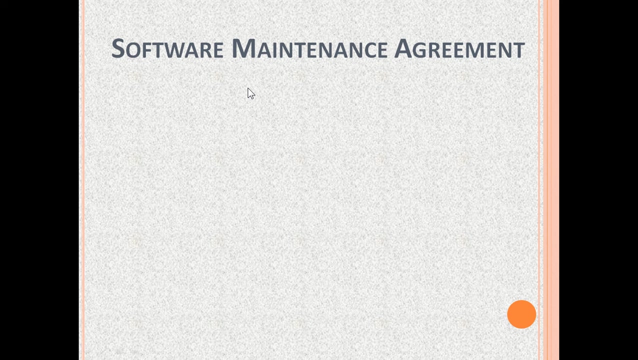 Making the software work in a new environment is called adaptive maintenance. Finally, software maintenance is also required to delete the retired functionalities. Now let us see software maintenance agreement. Now software maintenance is planned and agreed with the help of a software maintenance agreement. 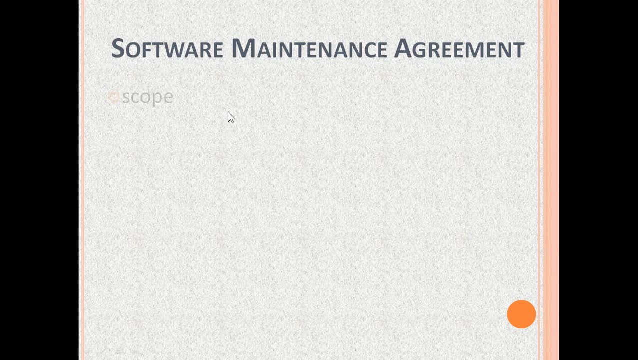 Now. this document states the scope of software maintenance. It also mentions transition. Transition means training from the software developers to the maintenance team, setting up help desk, etc. Service level agreements and incident management. Incident management means receive requests, log the requests. 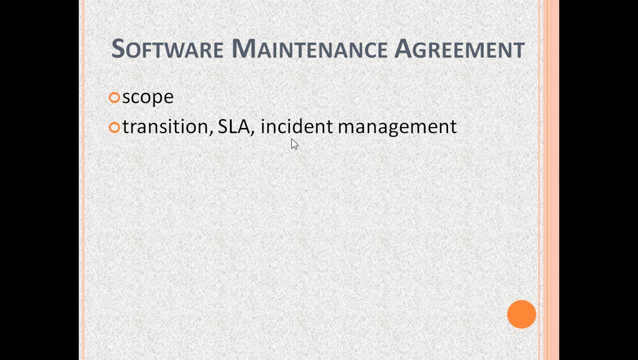 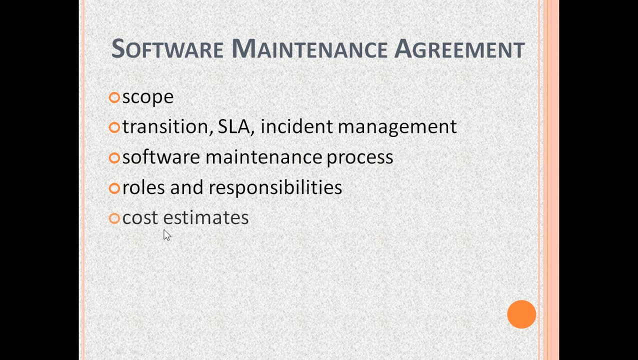 prioritize them, send them to the responsible role and track them until they are closed. Software maintenance agreement also mentions the software maintenance process. We will see this in just a moment: Roles and responsibilities in the maintenance team And cost estimates. Now let us see the software maintenance process. 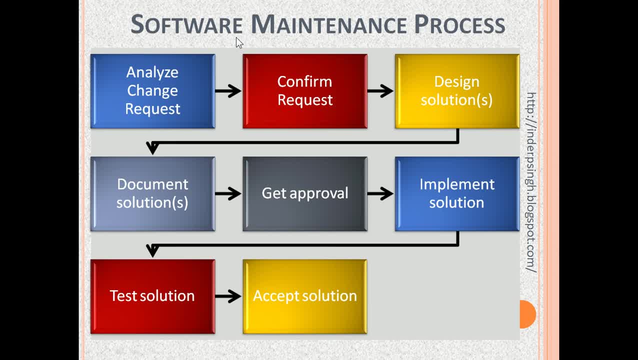 The software maintenance process is done by the software maintainers. It generally involves tasks like analyze, change request. confirm or deny the request. based on the analysis, design one or more solution options. document the possible solutions. document the possible solutions. then the users approve one of the solutions.